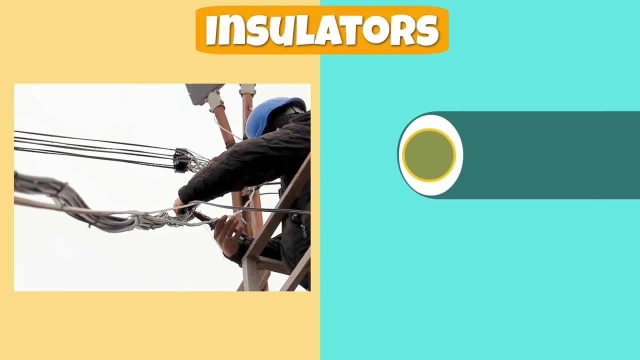 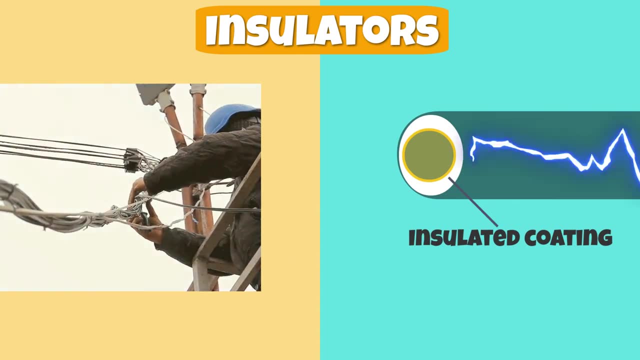 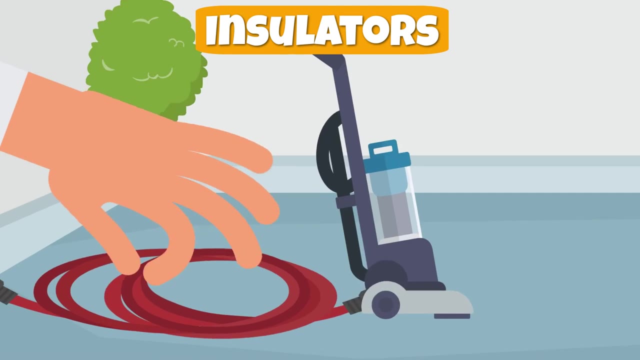 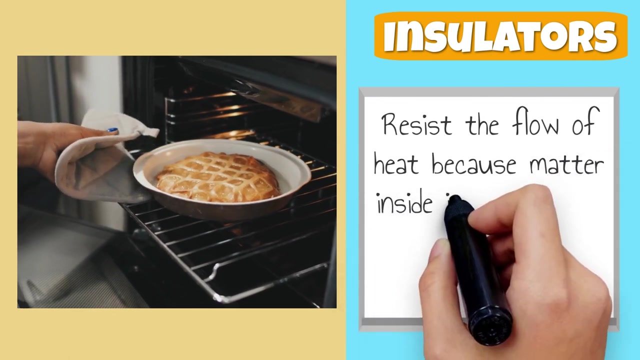 energy to escape. This is a perfect example of an insulator, because the energy that is used to control a part of the electrical entsteach is in the form of the material. They keep the heat. naturally. When you grab a wire that's properly coated, the electricity doesn't float from the top and they can06 ranked in advance with the right speed楚 down. See need to know how to extract when you want to enjoy 20ятm. Kendra미 masculi 여미 Music 804 Fernandez. the insulated coating resists the flow of electricity and keeps it in place. When you grab a wire that is properly coated, the electricity does not flow to you and shock you, and that's a very good thing. Insulators also resist the flow of heat because matter inside is arranged so that heat does not flow easily. When you go to order your favorite hot beverage, it will be handed to you in a styrofoam cup, ceramic mug or plastic Nachtem syf� 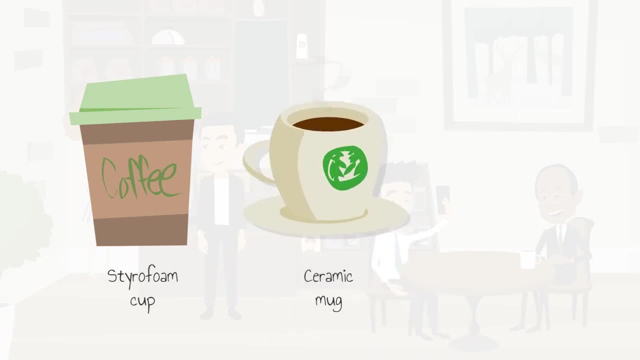 If you're with aboy and you're renewing the small cities, mayor, maybe you like the Requiem. thank you, styrofoam cup, ceramic mug or a cardboard sleeve, because they are all great insulators. They trap the heat from the coffee to. 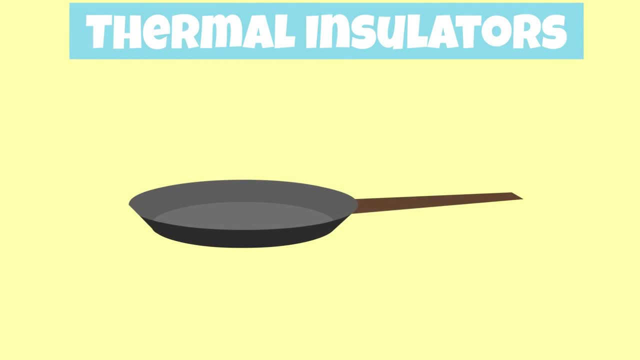 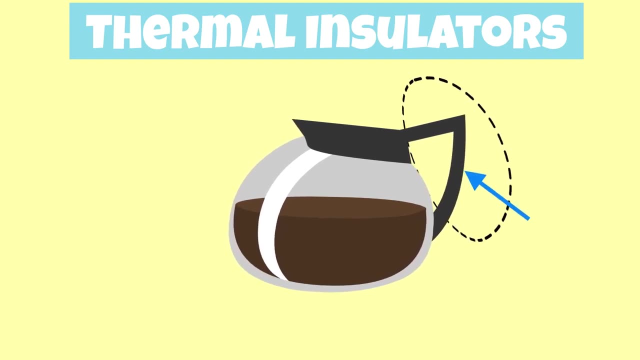 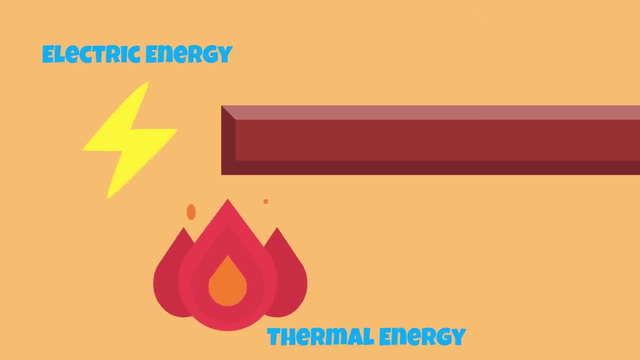 prevent you from getting burned. That's also why most pots and pans have plastic or wooden handles. The matter inside, the plastic or wood restricts the flow of energy, so it does not heat up. This is because when electric or heat energy flow through a conductor, the atoms move quickly and it becomes 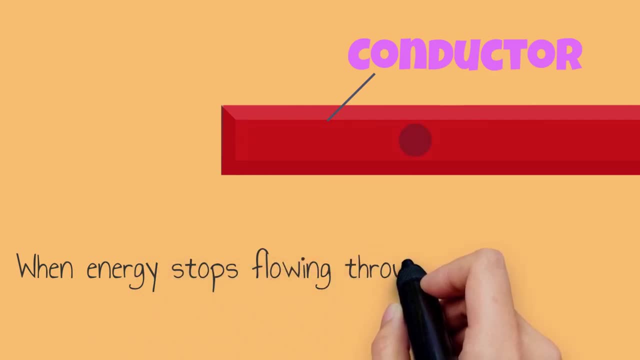 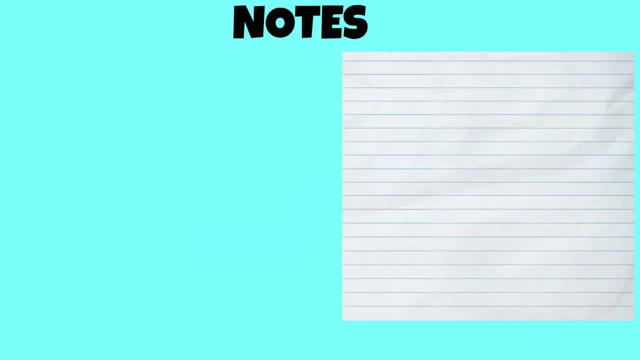 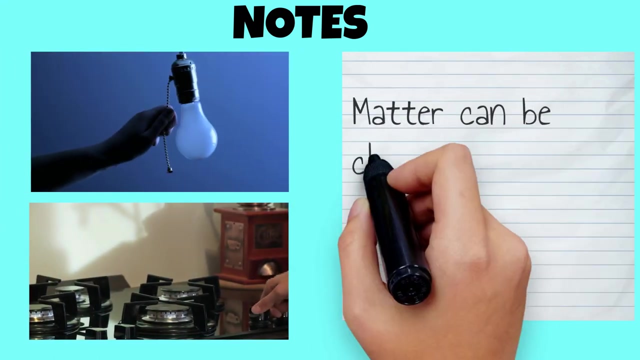 hot. When energy stops flowing through the conductor, the atoms slow down and it starts to cool down. Let's review what we learned. Insulators do not allow for energy to flow freely and it keeps the object cool to the touch. Matter can be classified. 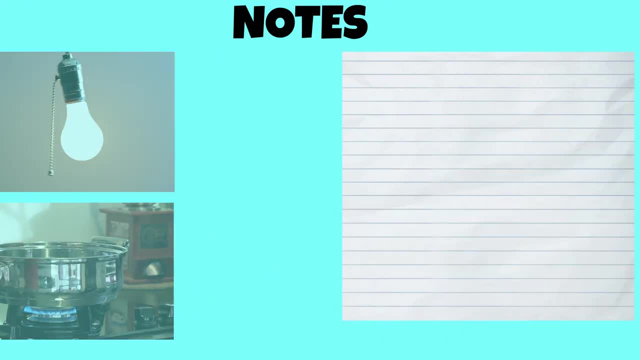 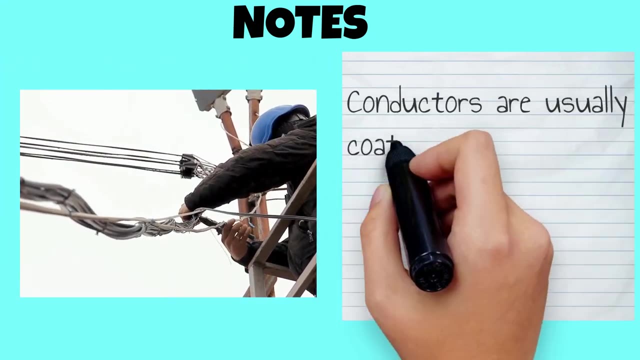 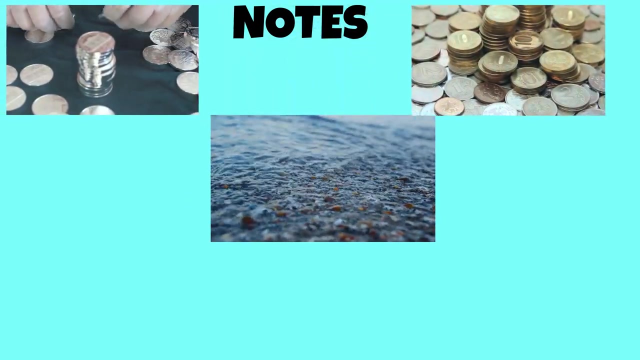 by its ability to conduct heat or electricity. The motion of atoms create and transfer heat and electrical energy. Conductors are usually coated or wrapped with insulators to contain the energy and protect us Seawater. silver, copper, aluminum and iron are all good conductors of electricity. 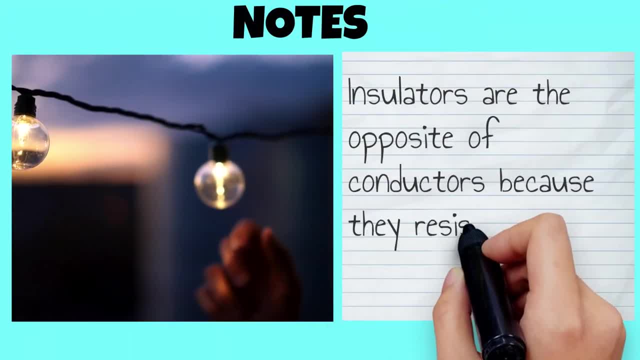 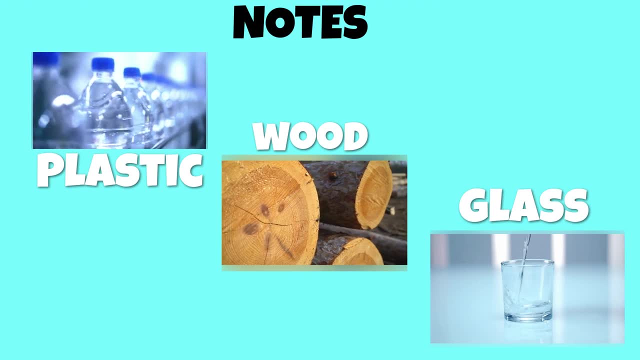 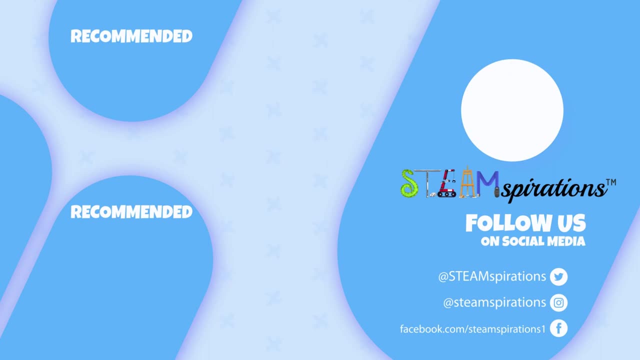 Insulators are the opposite of conductors, because they resist the flow of electricity or heat. Examples of insulators are plastic, wood and glass. Thank you for watching this video. If you have any questions, please post them in the comments.